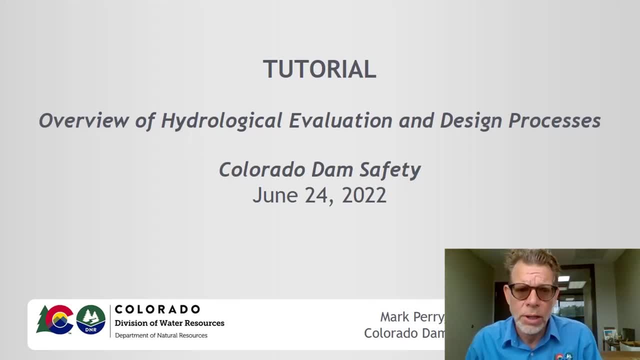 going with our hydrology analysis for Colorado Dam Safety purposes. So the easiest way I can summarize it is: we now have two processes. The first is hydrologic risk analysis: risk-informed decision-making for the evaluation of hydrologic adequacy for existing dams. Okay, that's the first. The second process is for design. 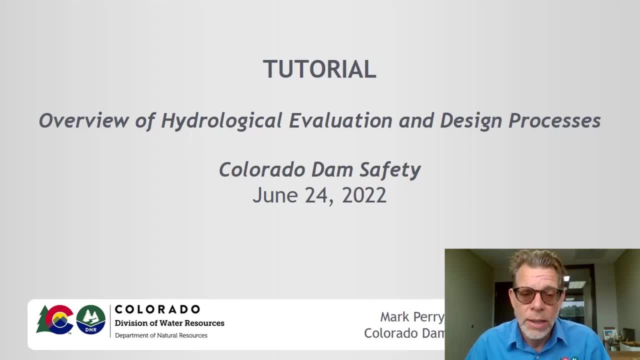 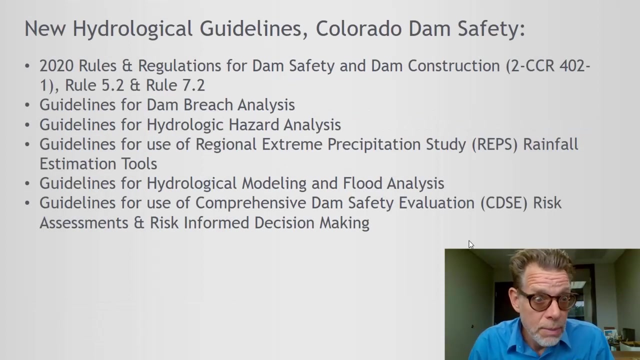 determining inflow: design, floods, IDF criteria, hydrologic hazard category to determine your IDF for use in design processes. So that's the first step for the project, for new dams raises new spillways and appurtenances. Okay, but first let's look at quickly at the various methods we have developed that the new, 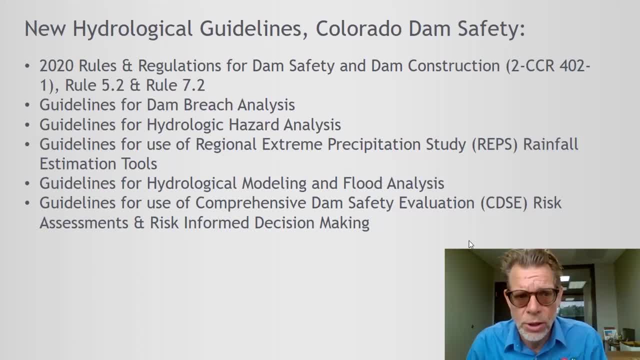 processes are built on And, like I said, we won't get bogged down into the details here. The details exist other tutorials and in the guidelines themselves, But let's just do a quick rundown. So, firstly, are we developed our 2020 rules and regulations? 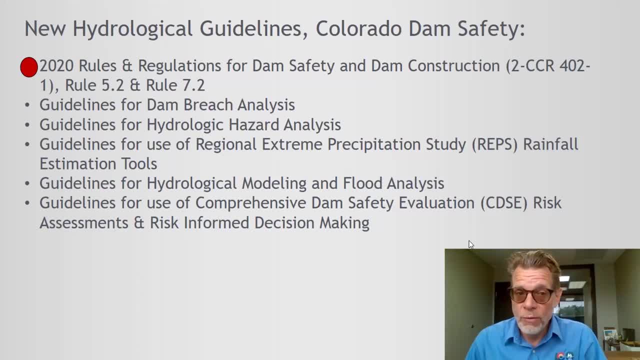 for dam safety and dam construction. Mainly, rule 5.2 is for the rule that covers the state engineer's safety evaluation of existing dams, which comes from our authority under statute 3787-107.. 5.2 lays out the rule for evaluating dams. 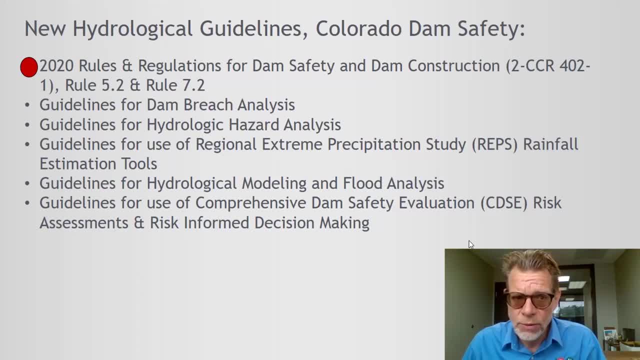 by potential failure mode analysis or risk analysis, risk-informed decision making. Then rule 7.2 deals with design standards. So rule 7 is design. 7.2 lays out the design standards. IDF criteria for hydrology, hydrologic loading. 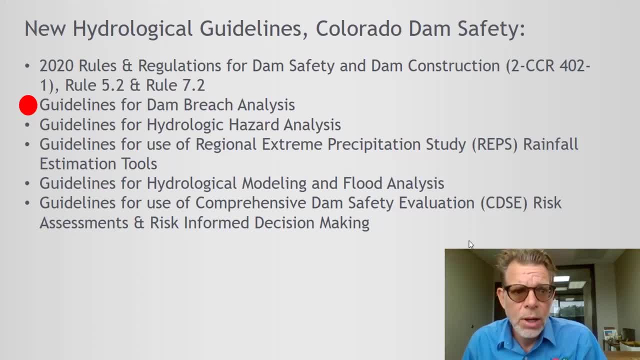 We also developed our guidelines for dam breach analysis, which you'll use in our guidelines for hydrologic hazard analysis. That's consequence analysis. We have our guidelines for use of a regional extreme precipitation study- REPS, rainfall estimation tools- and that feeds into 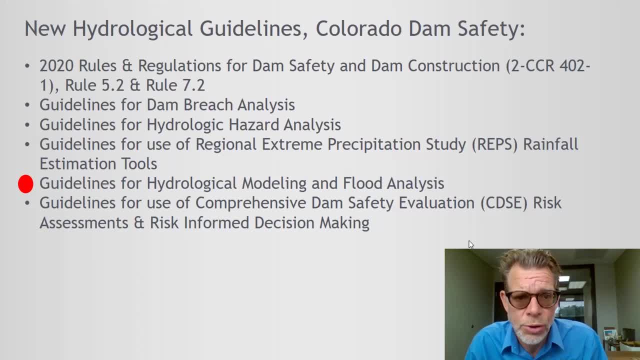 rainfall, runoff modeling, which is in our guidelines for hydrological modeling, flood analysis and finally, for the risk analysis, risk-informed decision making. That all feeds into our guidelines for use of comprehensive dam safety evaluation, CDSE, risk assessments and risk-informed decision making. 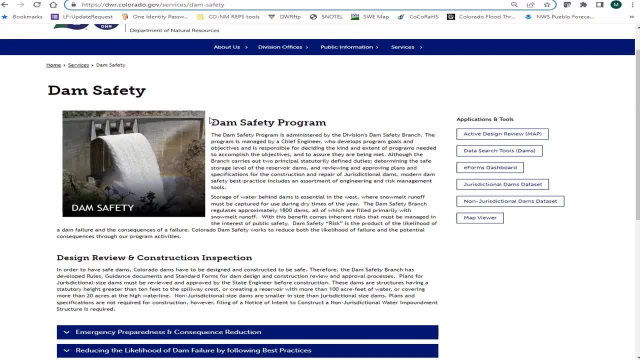 Okay, let me show you quickly where on our Colorado Dam Safety web page the various rules and guidelines, So that you can go to those find them, and then we'll get into this overview of our hydrological processes for evaluation and design. All right, so scroll, go to our Colorado Dam Safety. 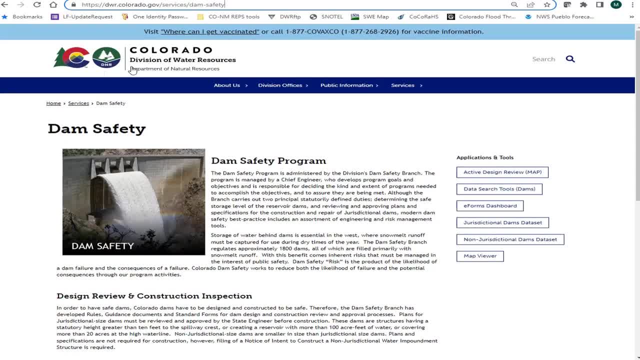 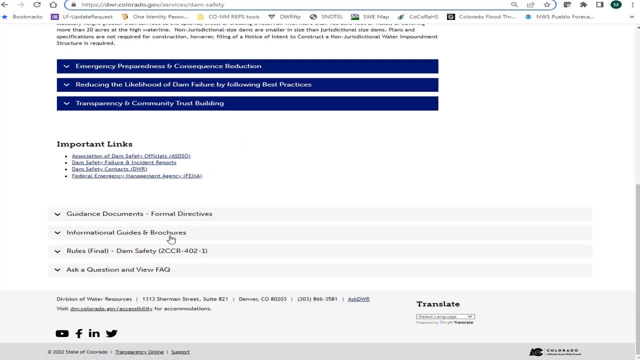 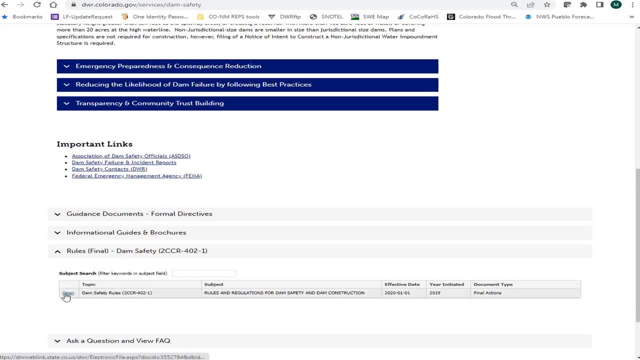 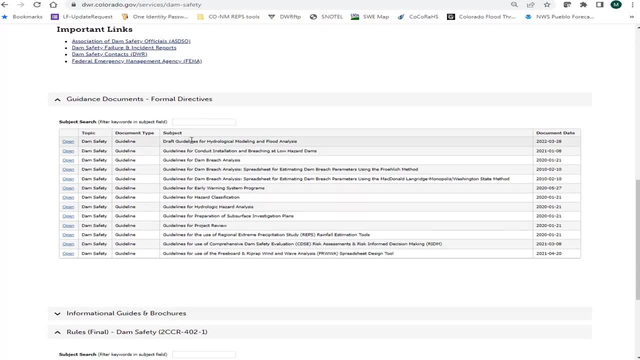 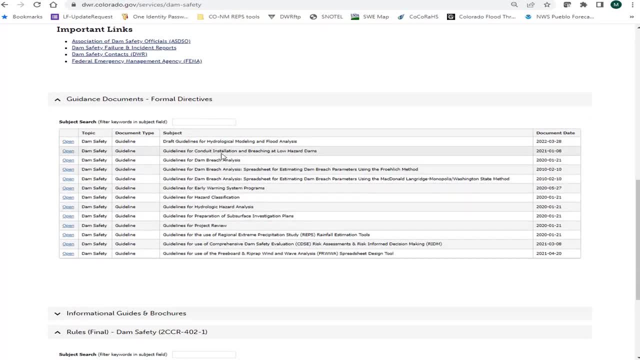 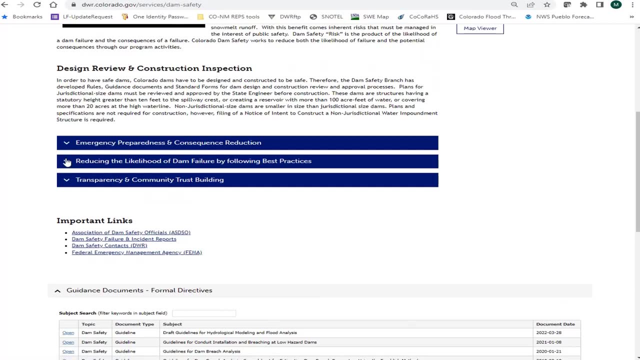 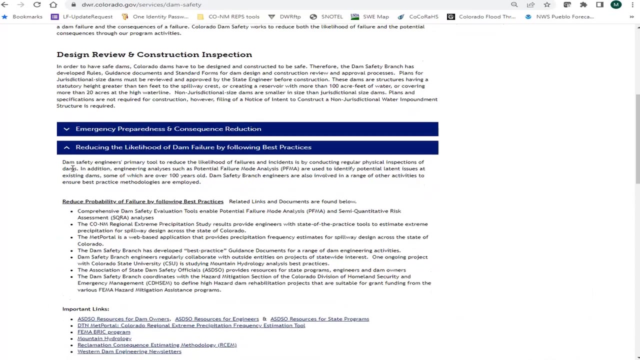 all the ones that I mentioned in the previous slide and a lot more. All right, and then up to the blue bars. we have reducing likelihood of dam failure by following best practices. So if you drop that down, there's a lot of interesting stuff in here, but 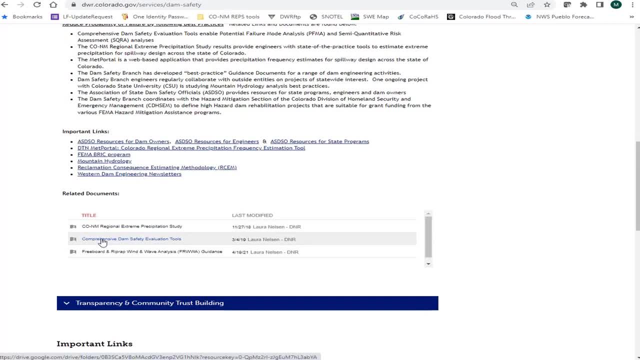 of interest to us here that we have an overview of hydrological evaluation and design processes document. that is the basis for the tutorial presentation here today And that is kind of buried at present. We'll try to bring it up more front and center, but for now you can find it under that blue dropdown. All right, and then we'll try to bring it up more front and center, but for now you can find it under that blue dropdown of reducing likelihood of dam failure by following best practices. All right, and then we'll try to bring it up more front and center, but for now you can find it under that blue dropdown of reducing likelihood of dam failure by following best practices. 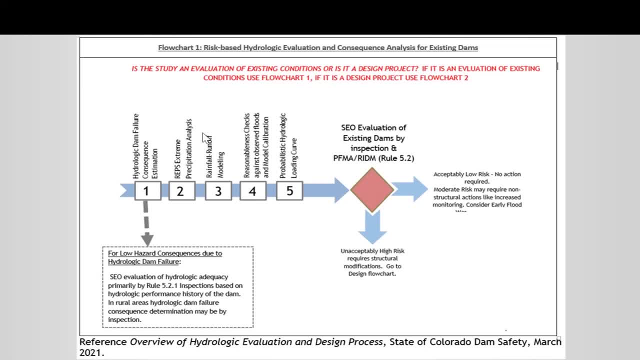 All right, and then we'll try to bring it up more front and center, but for now you can find it under that blue dropdown of reducing likelihood of dam failure by following best practices: annual exceedance probabilities one in 10, up through one in 10 million. And then there are three different storm types. So we have the two-hour local storm, the small intense thunderstorms, six-hour MECs- medium size, medium intensity- and then the long duration, 48-hour low intensity, MLCs or mid-latitude cyclone storms. Three storm types, seven AEPs, So that's 21 storms total. 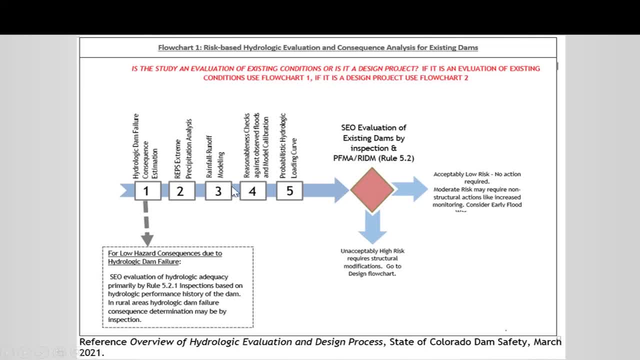 Get all those from reps, Run those through a rainfall runoff model, which is our CSU SMA method, And then we do the reasonableness checks. So we're checking the model to make sure agreement with the observed flood record with stream gauge, stream stats, peak flow envelopes. 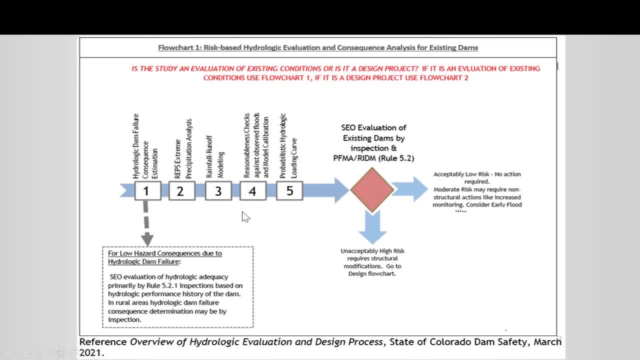 to get reasonable results. And that's all covered. steps three and four are all covered in our guidelines for hydrologic modeling and flood analysis. Once we're sure we have a model that's given reasonable results and defensible results, then we run all the reps- probabilistic storms- through the model and generate the peak. 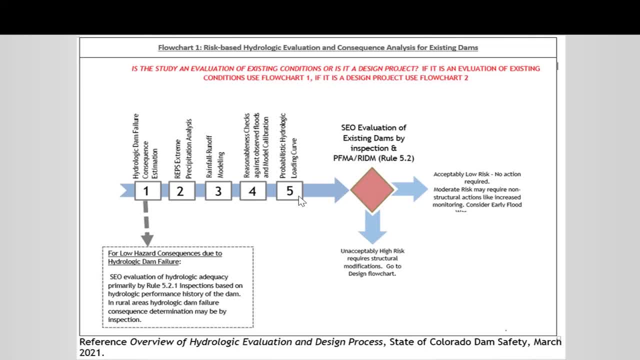 reservoir stages by AEP, which gives us a hydrologic loading curve, also called the reservoir stage probability curve or hydrologic hazard curve, And I'll show you an example of that. So now we have that, We have the consequence estimate from the hydrologic PFM. 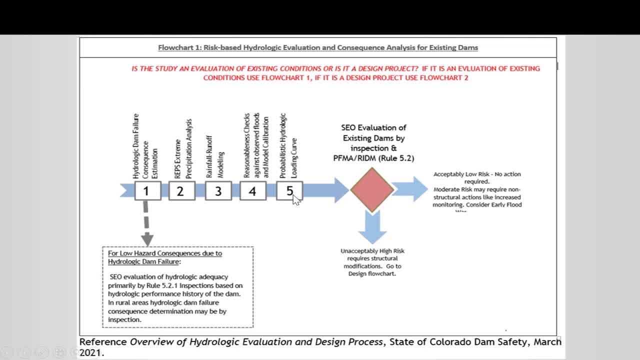 life-life estimate. and then we have the likelihood of hydrologic loading, And that feeds into our decision-making process, the hydrologic risk analysis, or risk-informed decision-making, where we, under state engineer, under rule 5.2, determines if the dam is. 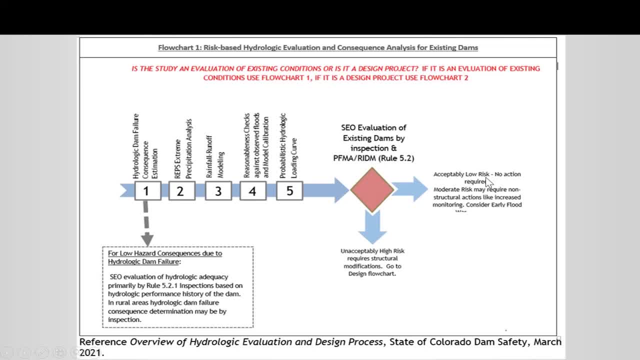 hydrologically adequate. So if the risk is acceptably low, no actions required. It's good, It's an acceptable risk under industry standards. If it's kind of moderate risk, there may be some non-structural improvements that an owner can make. early flood warning system. 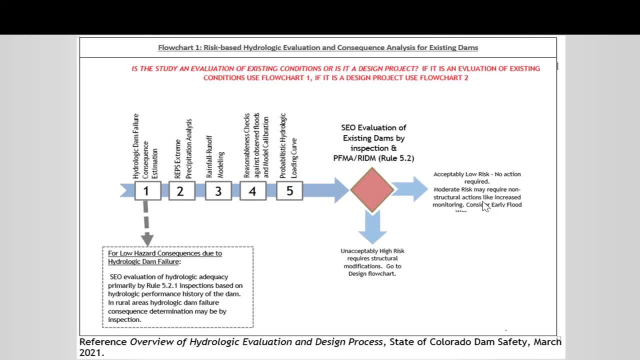 or emergency management, emergency action plan, type planning type of things to lower consequences. But if the risk is unacceptably high by industry standards, then we're talking about- we'd be looking at structural improvements to the dam and that would take us to flow chart, to 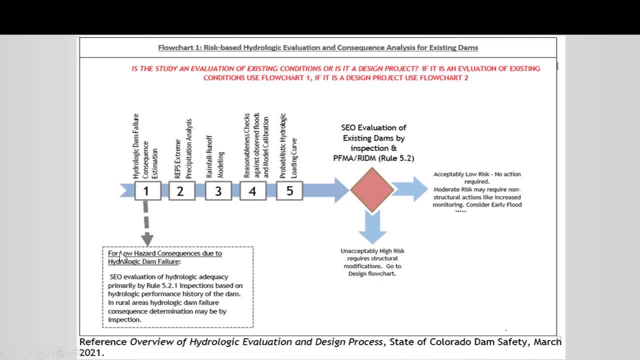 design standards, A couple of things before we get to that. So we have here in the gray dashed box a jumping off point. So if the dam is acceptably low, no actions required. So we have here in the gray dashed box a jumping off point for low hazard consequence dams. 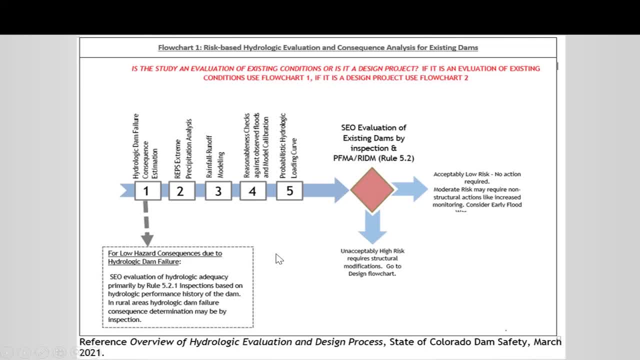 So if the consequences from hydrologic failure of the dam are can be demonstrated to be low, then we want to make this easier. We don't want it to be a put a bunch of owner resources or consultants or our resources into that. So if we can demonstrate low hydrologic hazard, 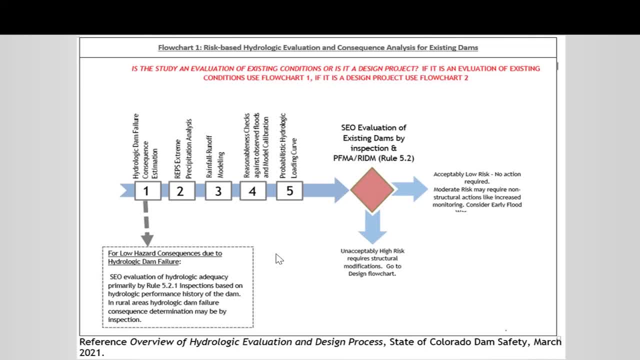 consequences. then we can evaluate the safety, hydrologic adequacy of the existing dam, Really just by inspection. And what I mean is looking at the performance history, the, the, maybe some rules of thumb, maybe stream stats or sizing, looking at the capacity of the. 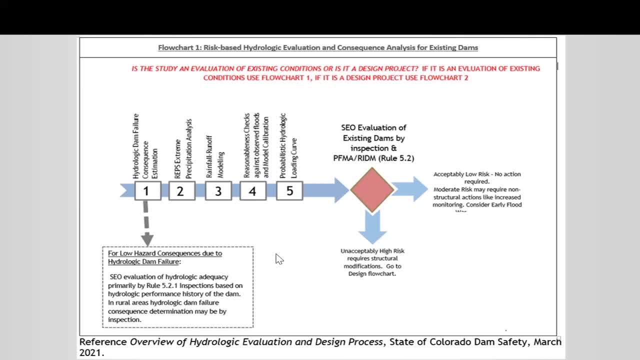 existing spillway but not not necessarily full blown risk analysis process for low, low hazard consequences from hydrologic dam failure. And we say that if, if it's in a rural area or just downstream rural land use or ag land use, then that high, low hazard consequences determination can be made by inspection. 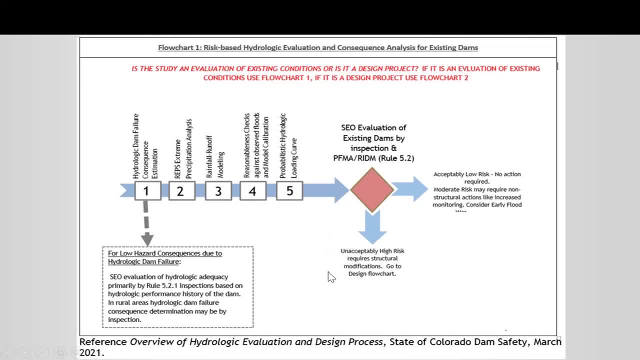 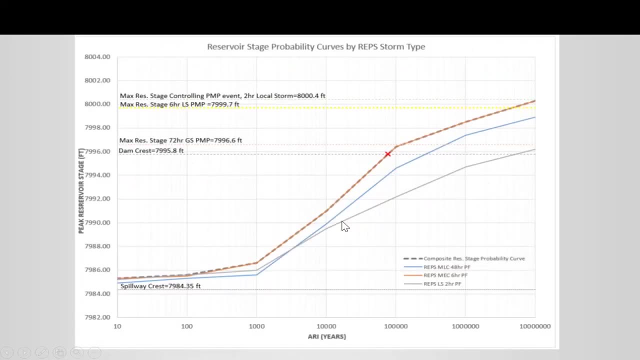 Okay, And so before we go to design, we're going to talk. I want to talk, walk through a couple of these steps in this risk analysis hydrologic risk analysis process. Okay, Okay. So the first here is the is the reservoir. 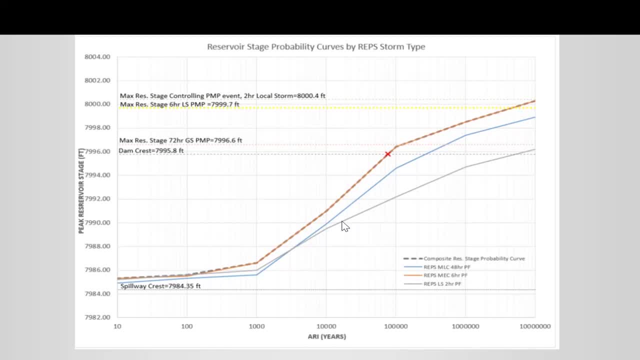 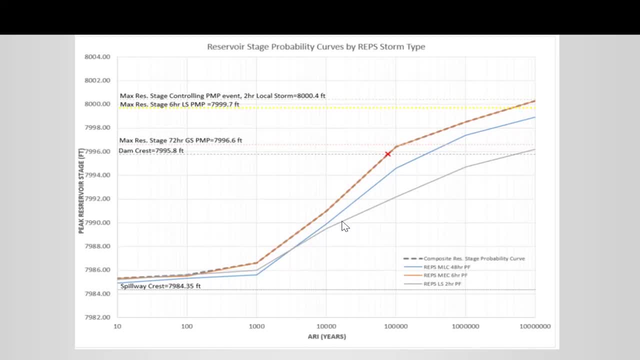 lifeless consequences from hydrologic dam failure. in that step one Now we go through the modeling, the reps- probabilistic storms, the modeling, and we generate these hydrologic hazard curves. Okay, So this is peak reservoir stage for each AEP storm and then the three storm types. 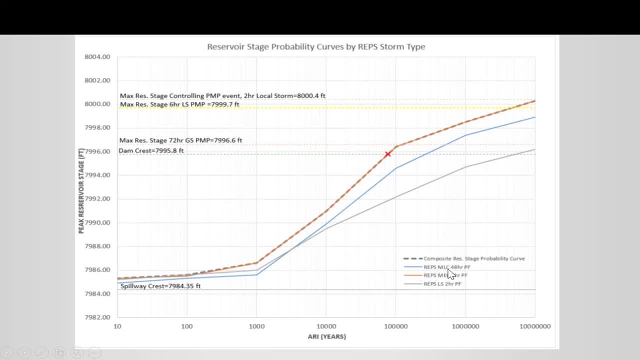 So here we're showing: the blue curve is the reps MLC 48 hour storms. the orange curve is the reps mec six hour curves. the gray one is the two hour local storms okay- and the controlling one. those can cross. they make different storms may control with different. 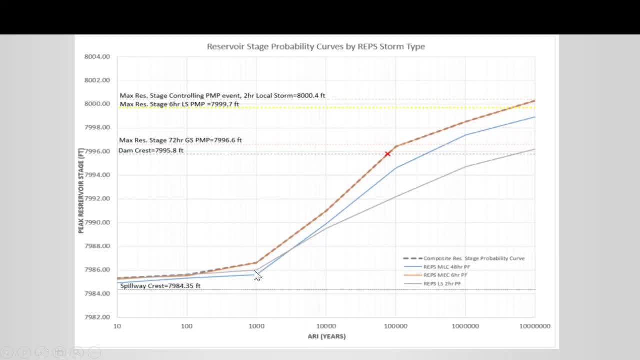 aeps, um, but the controlling uh upper line is the. the is what we call this composite or controlling reservoir stage probability curve. okay, um, here we've plotted reservoir stage on the y-axis and then annual recurrence or average recurrence interval on the x-axis, which is um, just the. 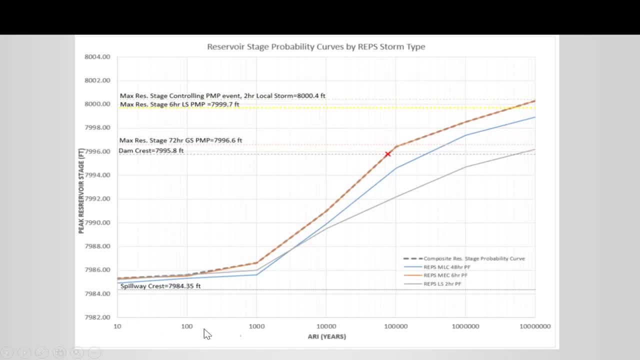 inverse of annual exceedance probability. so we're looking at 10 year, 100 year, thousand year, 10 000 year, etc. um, and then we can plot different uh key elevations as horizontal lines. the critical one here is the dam crest elevation and we're looking, we'd be looking at in this case, at 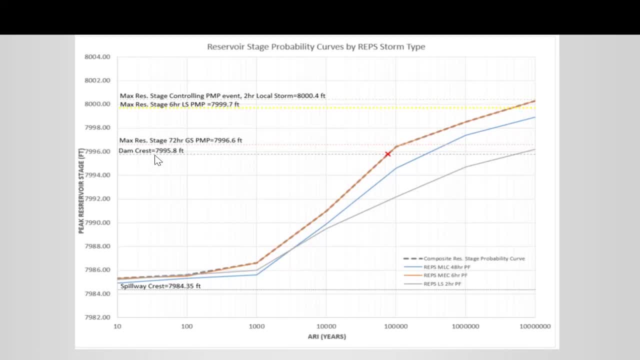 the overtopping uh, dam overtopping, pfm, and so we look at that controlling uh hydrologic hazard curve and where it, where it reaches the dam crest, that's incipient dam overtopping and we could call that the ari or aep of of um. 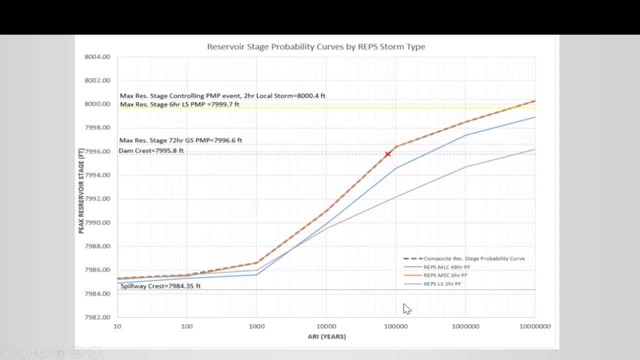 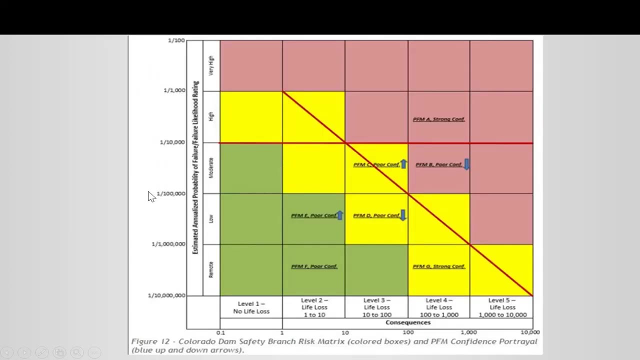 of the of dam overtopping. so in this case let's say it's looks like it's about 75 000 years, or for average recurrence interval, or an aep of 175 000. okay, the next, we take that, having determined that likelihood of critical hydrologic loading for the pfm um, so we, we go to our risk matrix. 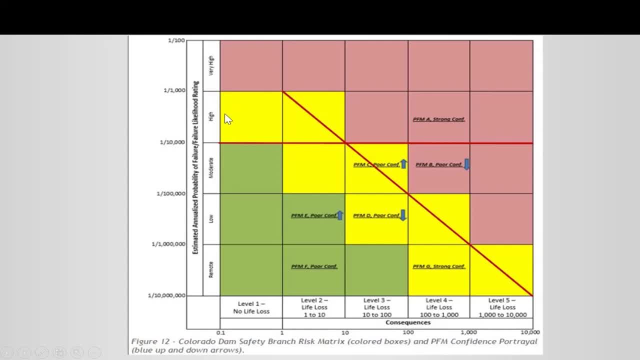 in um which comes from our colorado dam comprehensive dam safety evaluation, cdse guidelines, and we can plot uh that likelihood of uh hydrologic loading against the life loss consequences here on the x-axis. and so let's just say we were at life loss consequences of 50 and uh, uh likelihood of hydrologic loading of 175 000. we said so that. 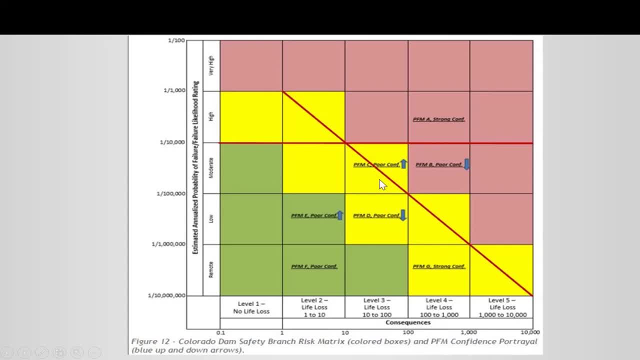 would put us somewhere, somewhere in here and the in the yellow square just below this diagonal red line, which is the societal um except societally acceptable risk line. so, like we said before, this kind of moderate area of risk, yellow may may allow, um may be acceptable to do some. 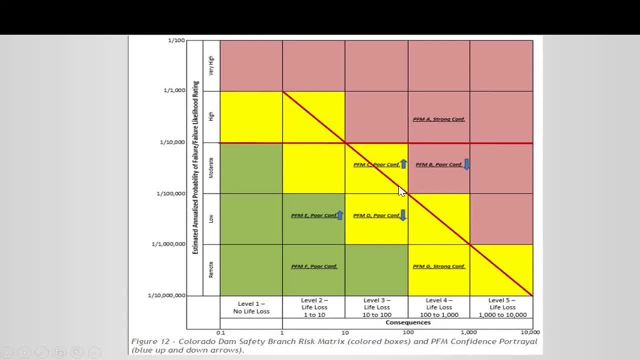 structural measures like an early flood warning system or better emergency planning to reduce consequences and get us to an acceptable level of risk. if we're down here in the green, if the risk plots hydrologic risk plots in the green, it's, it's okay, it's an acceptable level of risk by 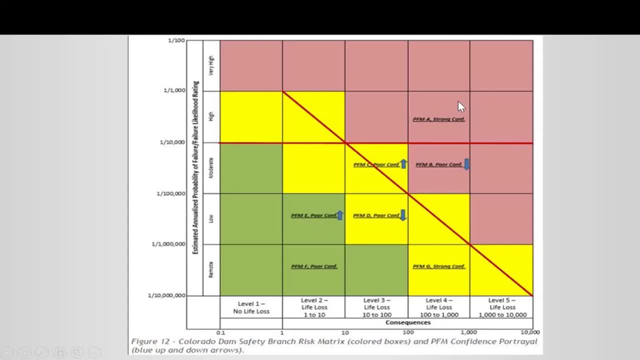 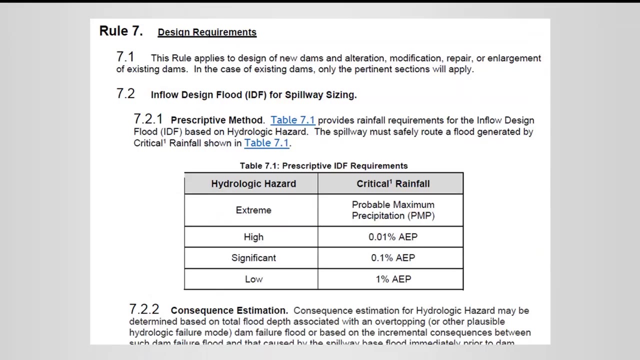 industry standards. but if we, if the hydrologic risk plots up here in the um red structural measures are going to be needed, most likely to um, reduce the risk, to um to an acceptable level of risk. um, if we continue to, may be going to say a later reviews of the existing apes. 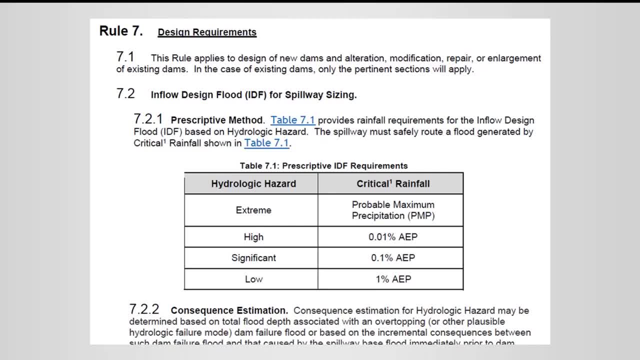 çocuğ um, how is the lunch if they do perform at least apes as intended, as just going over here closely or we're having a reallyître? the processes i want to look at second slide here will tell us about the idea that we can then se tempt in this turn for walking all the way up to. of feet stickingveland. okay. so now let's go to the hydrologic design process. so this is- i know this is the part that everyone WANTS to go to- that we're design engineers, we want to design and build things and we kind of automatically jump to the inflow design fund. but that first step for working on any existing dams, that first step of evaluating hydrologic adequacy by hydrologically adequate water fillglayner. 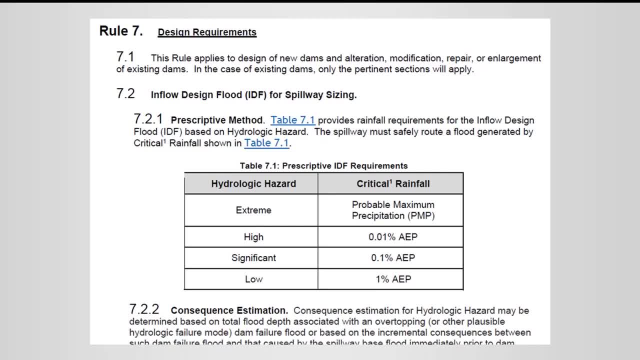 hydrologic risk analysis is critical And I want to reiterate that that determination comes from this. determination of hydrologic adequacy comes from the state engineer under rule five and statute. Then, if we're talking about existing dams, if we determine the dam is inadequate or 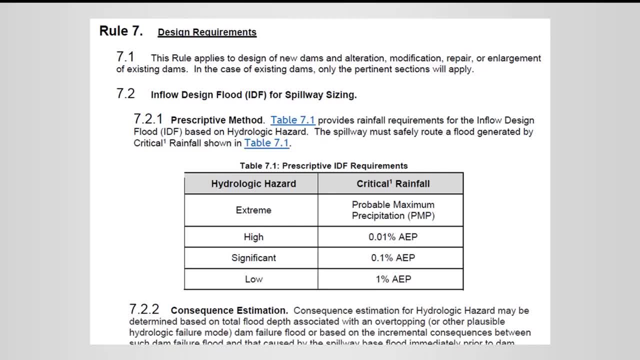 an actionable level of risk, then we go to design. Otherwise, you know you can, you might be going straight to design for a new dam, dam enlargement or any other modification, say for spillway modification due to concrete deterioration or condition, anything like that. So any 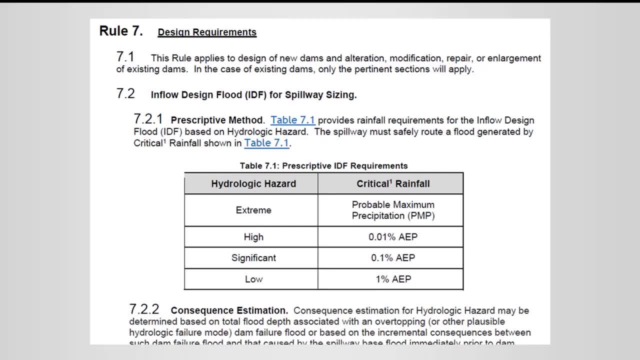 design process where we're going to design and construction will be this or any design project we're going to design and construction will be in a second process of determining inflow- design flow. So let's look at rule seven in our 2020 dam safety rules. 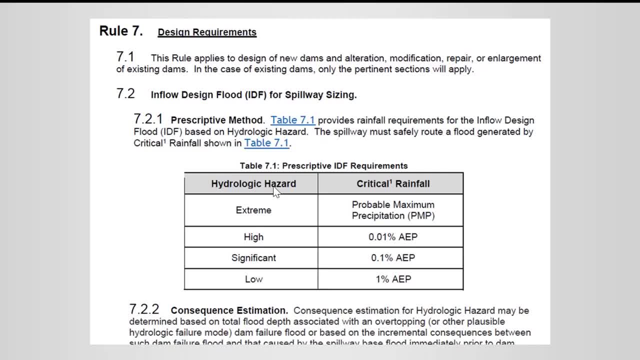 Rule seven two gives the criteria for inflow design floods. We have this hydrologic hazard category. We determine that by hydrologic hazard analysis and then we group the consequences into one of four categories- extreme, high, significant low- and assign a corresponding critical rainfall for the inflow design flood criteria. So extreme: 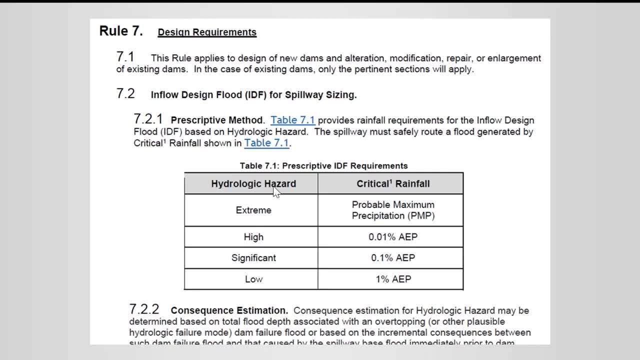 hydrologic hazard has a has a PMP storm or PMF flood. High hydrologic hazard has a 10,000 year flood. significant hydrologic hazard has a 1,000 year flood and then low hydrologic hazard has a 100 year, 100 year flood. So from and these 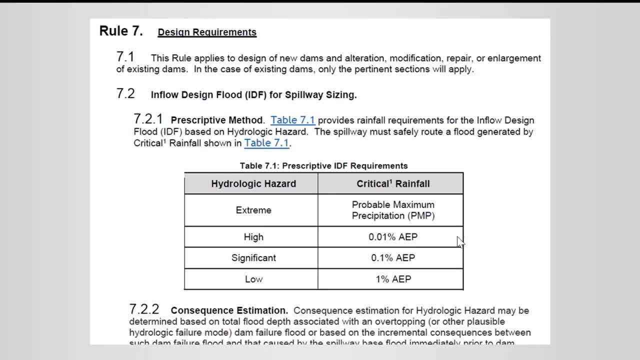 come from generally, come from the reps, our reps- rainfall estimate and then rainfall runoff modeling. So these are, these are hydrologic. the hydrologic hazard category is based on consequences from hydrologic dam failure, Again generally talking about earth dams, generally talking about overtopping dam failure. 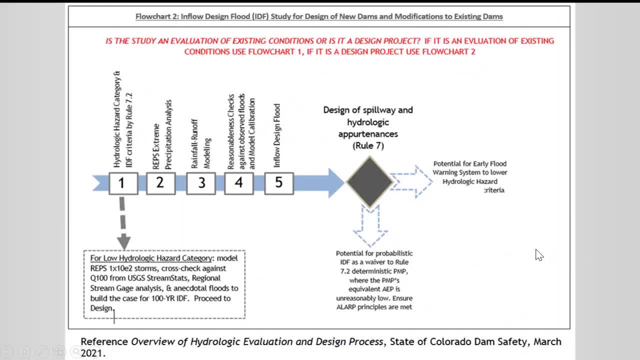 All right. so let's go to flow chart two, which goes through this process of design, determining an inflow design flood for hydrologic design. So flow chart two across the top: inflow design flood study. If you're doing an inflow design flood study, 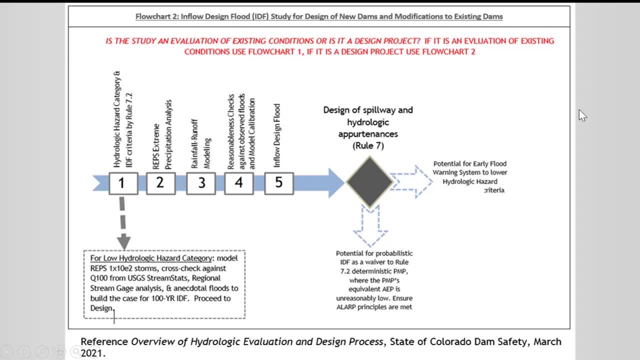 you're going to be doing this study for the design of new dam or modification to existing dams. Again, the big red letters at the top is a study and evaluation of existing conditions and existing dam, or is it a design project? If it's a design project, use this flow chart. flow chart two. 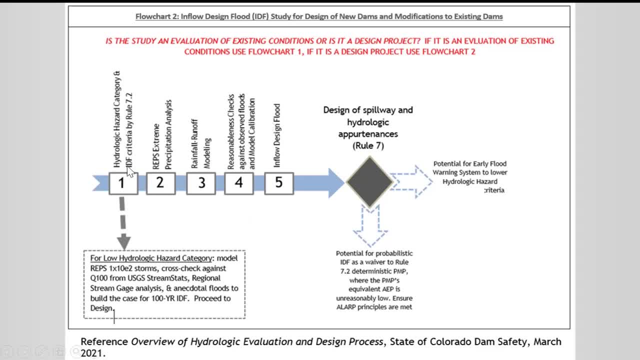 Looks very similar to flow chart one, but there's a couple of key differences. Now, first one: we're going to still going to do a. it's all still based on consequences- consequences from hydrologic dam failure- But in this case, 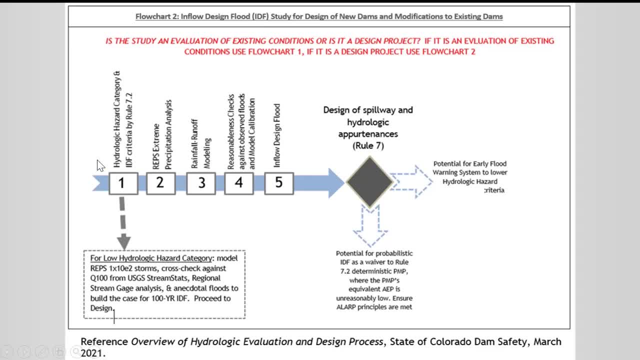 we determine. we use the our hydrologic hazard analysis guidelines. your reclamations are some method estimate life-loss consequences, or we can. we can also determine non-life-loss consequences at the same time, And then we group those into a hydrologic hazard category for purpose of determining the IDF criteria. 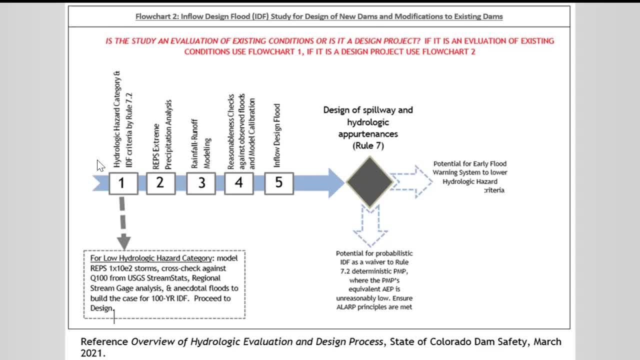 The categories are discussed in our rules, in rule seven two and in rule four, But again they're extreme, high, significant and low. The purpose of the hydrologic hazard category is to give us the to set the IDF criteria. 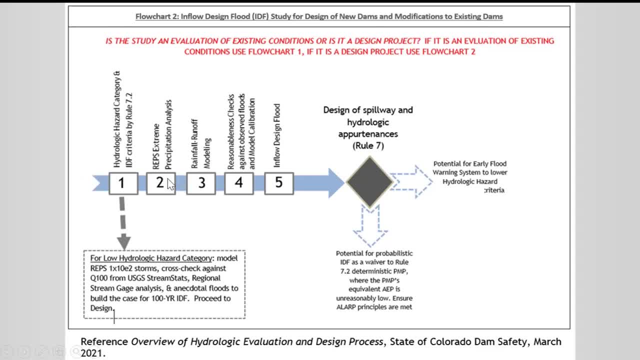 Then you model that, get your IDF criteria. model that storm in or, I'm sorry, do the rainfall analysis for that storm in reps. model that in our rainfall runoff. model our CSU SMA method, And then we still need to do all the reasonableness checks. 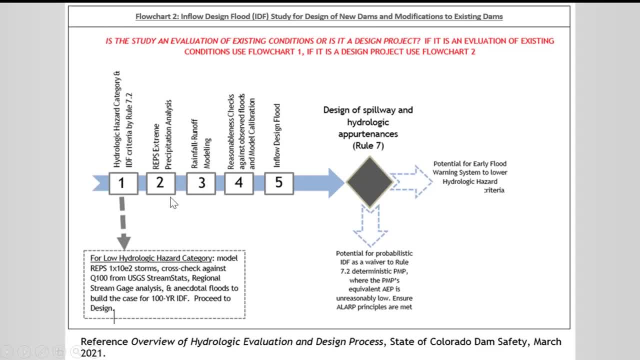 So you're going to still have to model other rep storms to do the reasonableness checks, to check against stream gauge analysis, to check against blue sky, frequency, floods, stream stats, peak flow envelopes, to make the case that the CSUSMA. 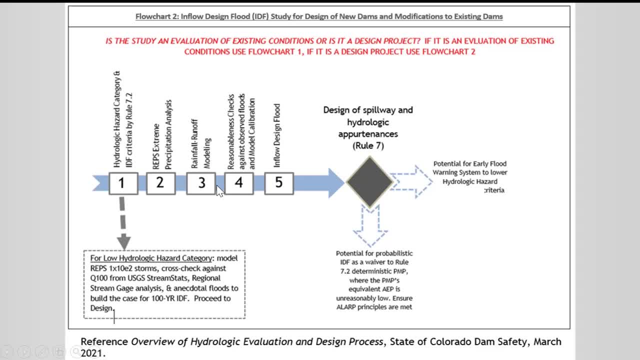 model is giving reasonable results. We want to have reasonable inflow design floods, just like we want to have reasonable floods in the hydrologic risk analysis. So once we've made the case against the observed flood record that the model is giving reasonable results, we can use the inflow design flood that comes out of the model So that then we carry into. 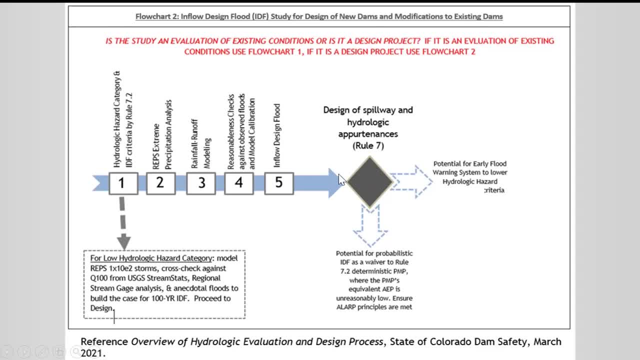 your decision-making step, if you will, basically your design. So design a new dam, enlargement, modifications per the design standards and rule seven. So we have just a couple kind of qualifiers here. I guess with the dashed arrows There is still potential for. 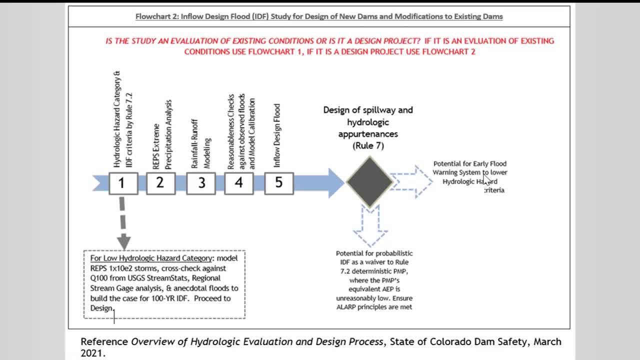 early flood, use of an early flood warning system or improved emergency action planning to lower life-loss consequences. Going back to step one, there is that could be used to lower hydrologic hazard category, which would in turn lower your IDF criteria. And then this bottom arrow, what we've seen. 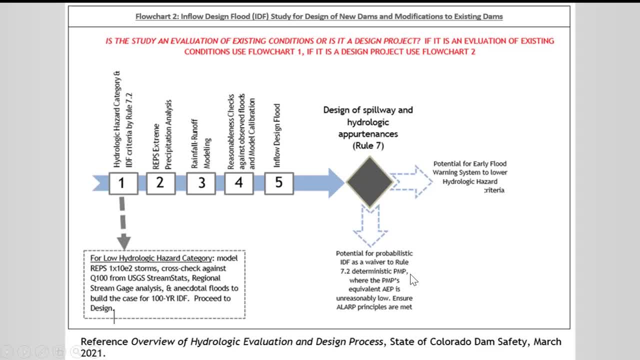 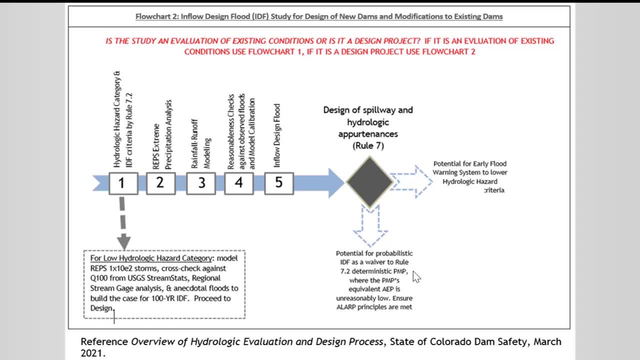 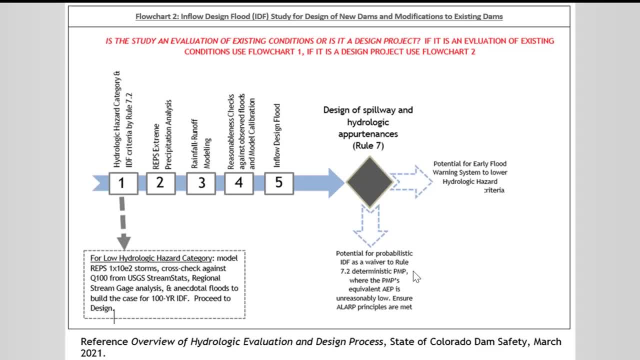 for dam safety. So what we have done is that we have the possibility of, in that case, of granting a waiver- a state engineer-approved waiver- to the PMP IDF criteria and substituting a lower risk-based IDF criteria. in that case, All right And as we had, 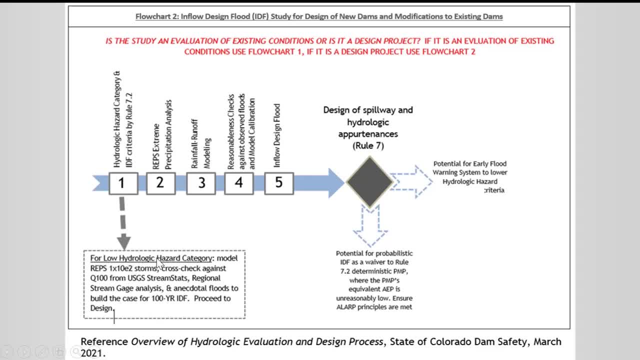 in flow chart one. again, we have a jumping off point for low dams with low hydrologic hazard consequences or low hydrologic hazard category. So again, we want to make this simple, in this case as simple as possible. We don't want to use owner and consultant and our resources. 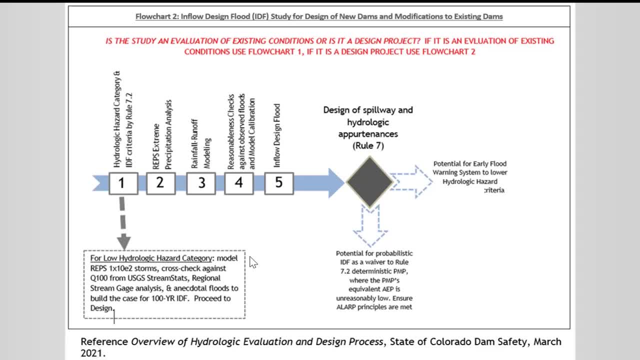 on low hydrologic hazard. So we want to make this simple, in this case as simple as possible. excessively on waste resources on low hydrologic hazard dams. So the simplifications here could be just using it's the IDF criteria is a hundred year storm, hundred year flood. So we could just 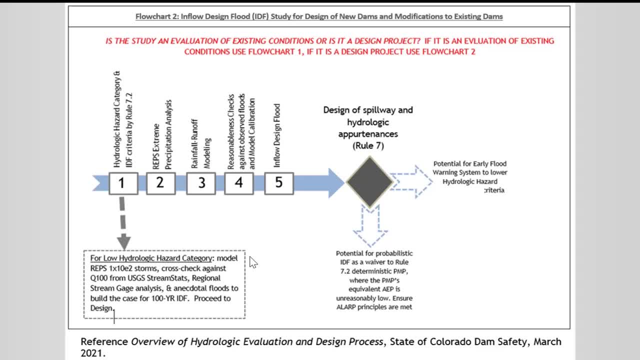 go straight to using stream stats or if we have a stream gauge, a flood frequency estimate, to get a hundred year flood. And if you want to just design this spillway to pass a peak flow, then that may be it. Now, if there's significant, if you expect. 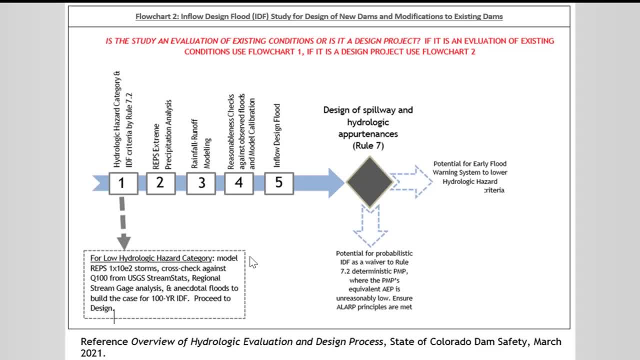 significant reservoir routing from a good size reservoir, then you may still want to do the modeling. just compare the model to the hundred year, calibrated in that way, And then you would and then do your, use your model to you do reservoir routing, But we want to keep that. 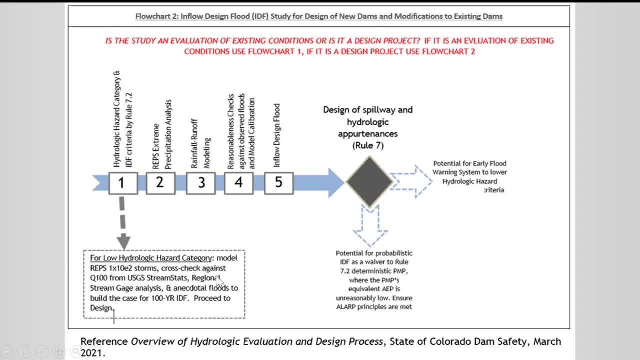 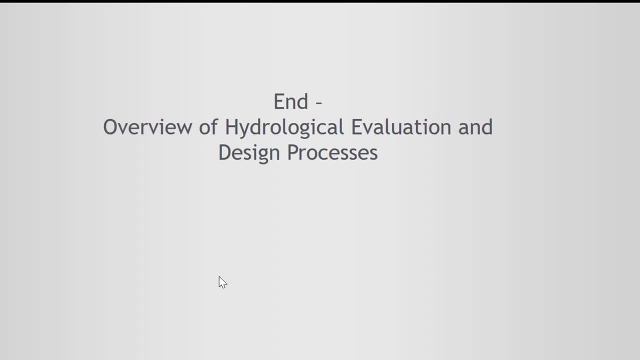 process simple for low hydrologic hazard category dams. Okay, That's the end of the overview of hydrologic evaluation design processes- two main processes. Let's just recap what we talked about. Two main processes. The first, hydrologic hazard analysis. for the evaluation of hydrologic 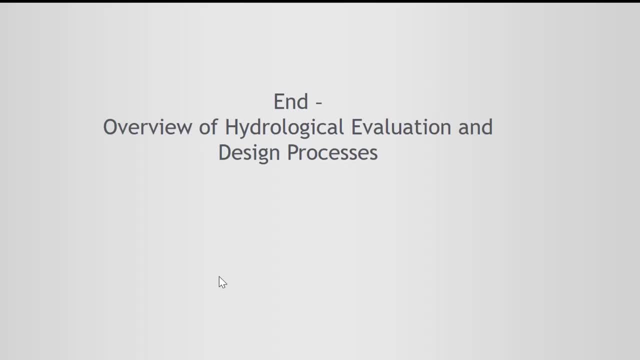 adequacy at existing dams. That's done by risk. in that hydrologic risk analysis, risk-informed decision-making, We get consequences: life-loss estimate and likelihood of critical hydrologic loading- We plot those on a risk-informed decision-making. We get consequences: life-loss.